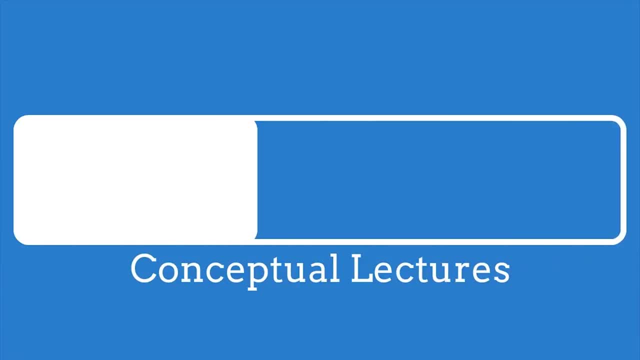 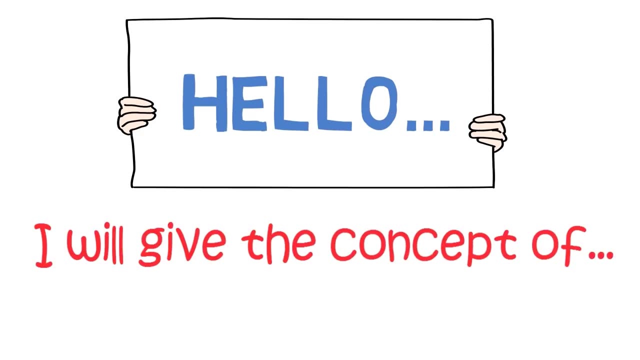 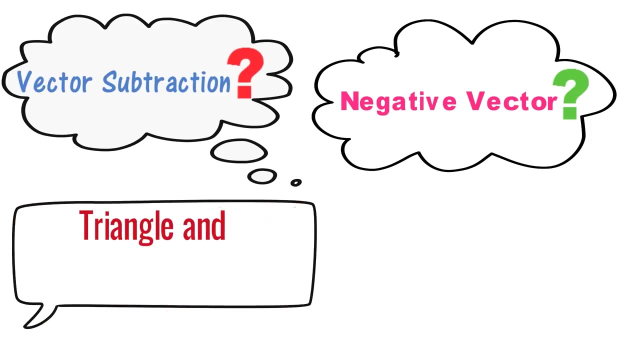 Hello. I will give you the concept of vector subtraction and the related topics: What is vector subtraction, What is negative vector, Vector subtraction by triangle and parallelogram law, And why vector subtraction is not commutative. And in the last of this video I will give 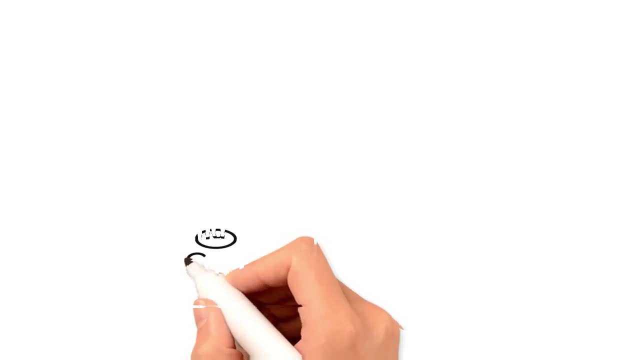 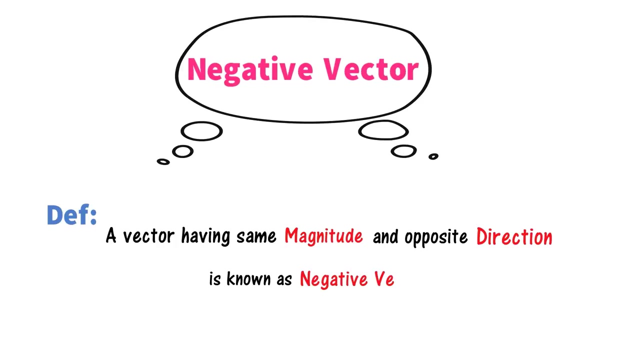 you the application of vector subtraction. Before telling you about vector subtraction, let me tell you about negative vector. The definition of negative vector is: a vector having same magnitude and opposite direction is known as a negative vector. Negative vector is also known as a additive inverse. Now, for example, if I have a vector A in this, 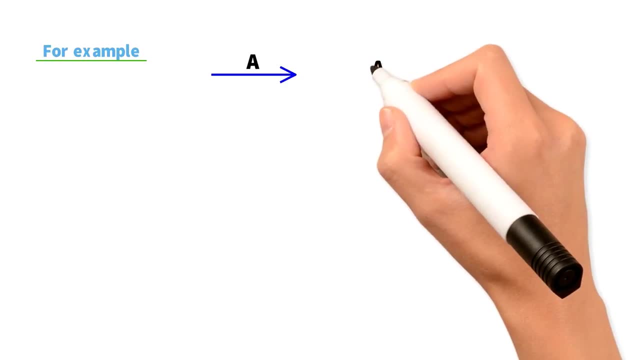 direction And let the magnitude of the vector be negative. The magnitude of the vector A is 5 units. Now if someone is asking me to find the negative vector of A, or if someone is asking me to find the additive inverse of vector A, then 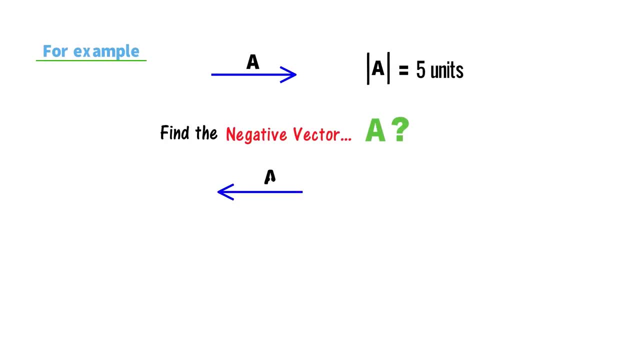 what I will do. I will just change the direction of the vector A and I will get minus A. Remember minus sign indicate the opposite direction And I will get. the magnitude of the vector A will be remaining the same And that will be negative unit And again, minus sign is telling me that this is in the 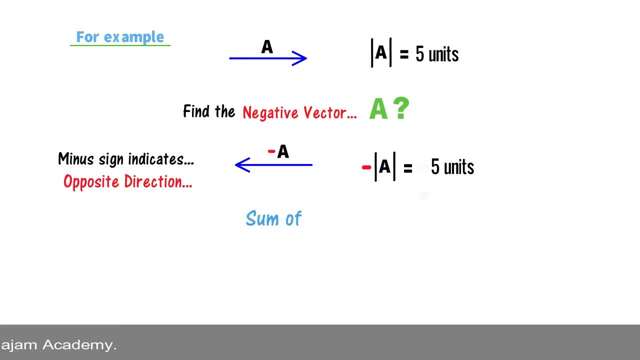 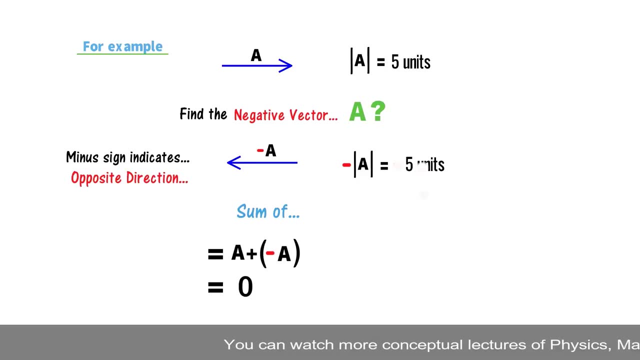 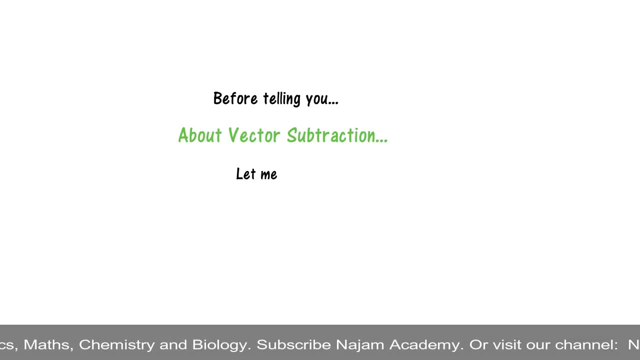 opposite direction. And remember: the sum of A plus minus A is equal to zero, because minus plus A and minus A will be cancelled out And I am getting zero and I am getting null vector. Before telling you about vector subtraction, let me play a part from my video. 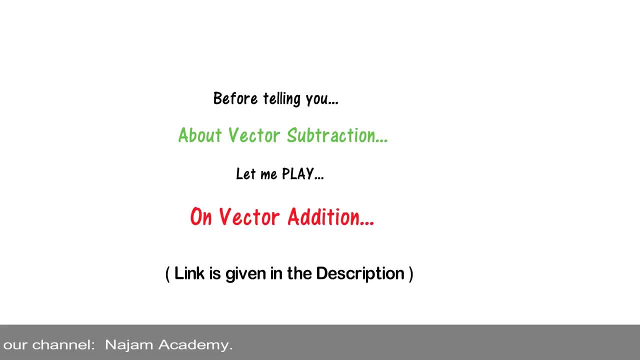 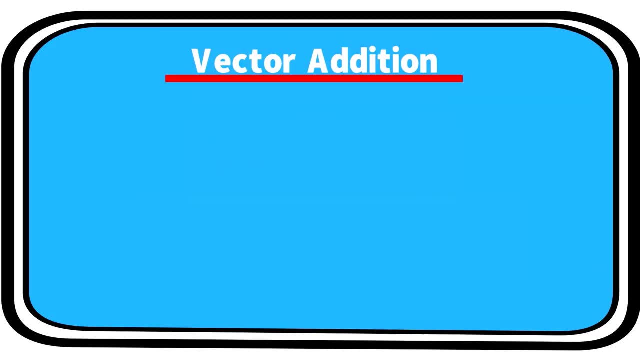 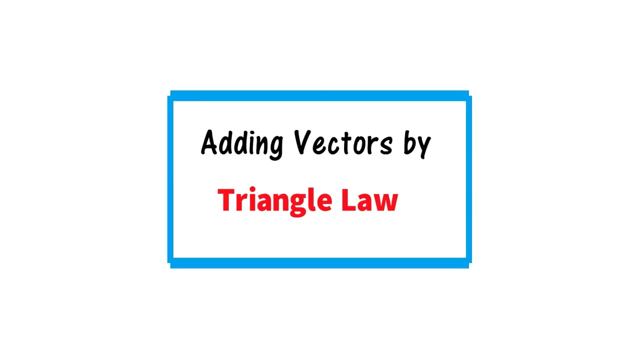 on vector addition. Now let me tell you about the addition of vectors. We can add vectors by two different law: By triangle law and by parallelogram law. Now, adding vectors by triangle law. Before telling you the concept of triangle law, let me tell you the tricky concept of 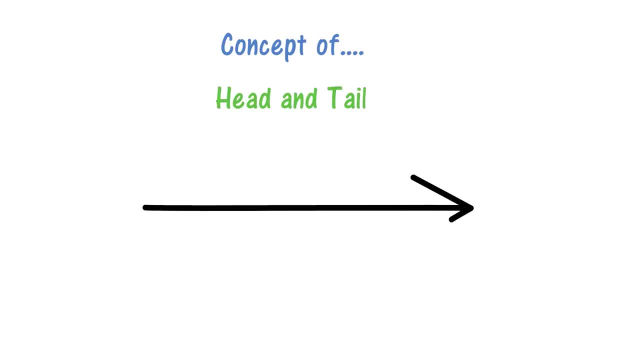 head and tail rule. Now, if I draw a vector, Now this part of the vector is known as a tail of a vector And this part of a vector is known as a head of a vector. Now, for example, if I have a three vectors: vector one, vector second and vector third- Now here, if I 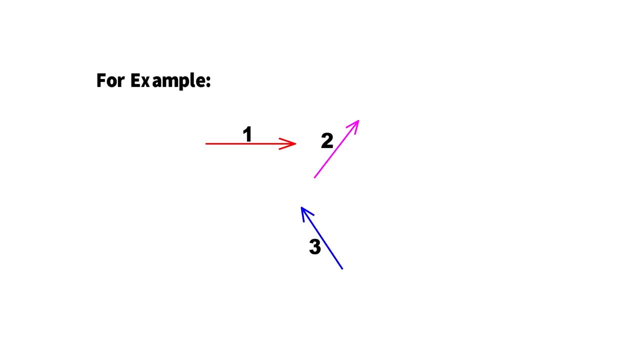 want to add these vectors. Before adding the vectors, I will join these vectors for the addition. Now how I will join these vectors for the addition. Now to join different vectors for addition, I am going to give you a trick And remember. 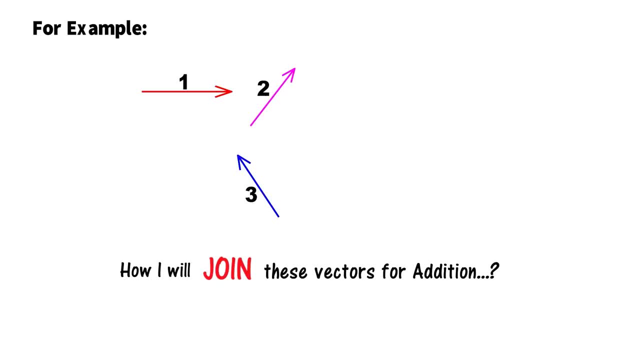 this trick wherever you are joining vectors for addition, And the trick is very simple And that is head and tail trick. What I will do. I will take the first vector Now, I will take the second vector and I will join the tail of the second vector with the head of 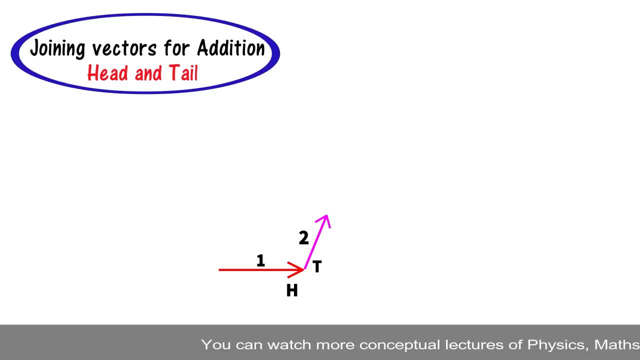 the first vector And then another vector. I will take the third vector and I will take the tail of the third vector and I will join the tail of the third vector And again this will come as a host number 2 vector. Now for each of the two vectors, I will take both. 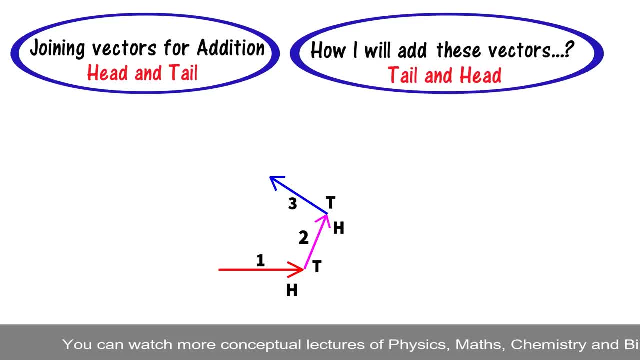 of these vectors. This is because there are numbers at the beginning of the head of the second vector And I know that I will toss point of each of the vectors to the first number. Now, in any case, take the first vector, a value, I will toss, and take the tail and the forming. 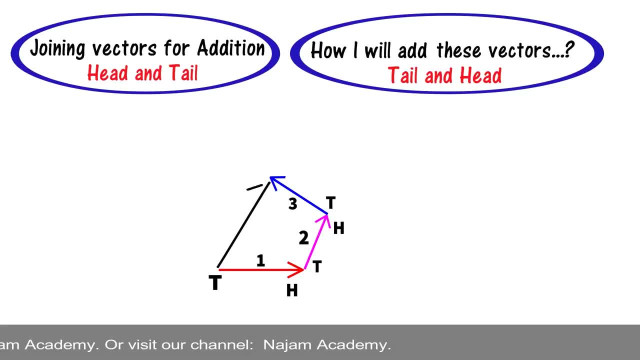 vector 2.. Now, if I want to join this other vector with the head of the last vector, and I will take the tail of the third vector, And now I have to join this head and tail, the head of the third vector, and this is the resultant vector. this resultant vector is actually: 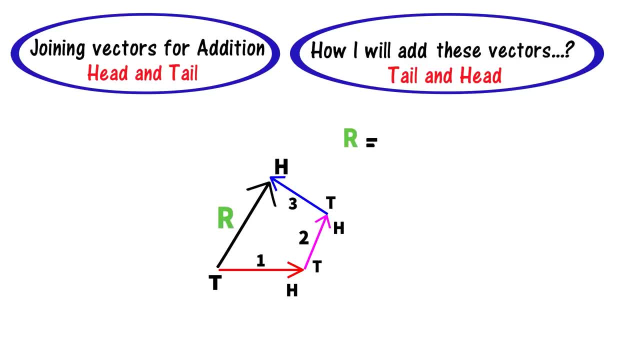 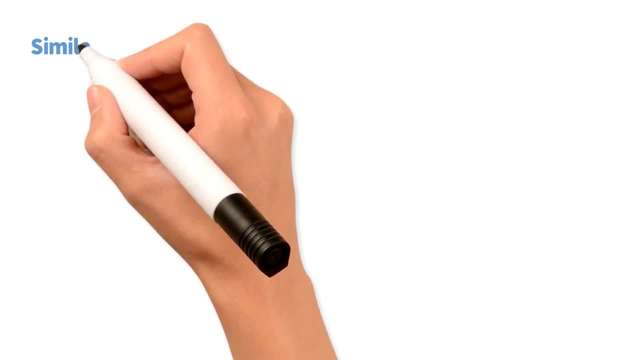 giving me the addition of these three vectors, one plus two plus three, and remember resultant vector is a vector which gives the result of all these three vectors. let me tell you about vector subtraction. similarly, if we have two vectors, a and b, and if someone is asking me, 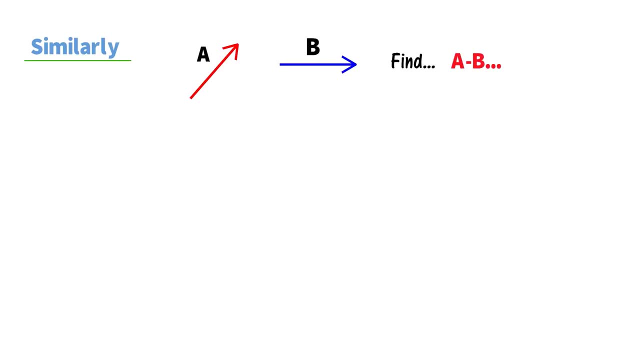 to find a minus b. now remember, here i need minus b, or i need the negative vector of b, or i need the additive inverse of b. so i will take the negative vector of b. is like this: now i can find the subtraction of two vectors by two different law. 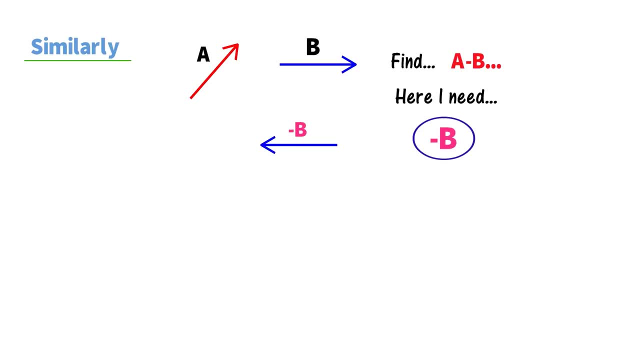 now i can find the subtraction of two vectors by two different law: by triangle law and by parallelogram law. now, here first of all, i will find the subtraction of a minus b by using triangle law. now, first of all, i will take the vector a and then i will take 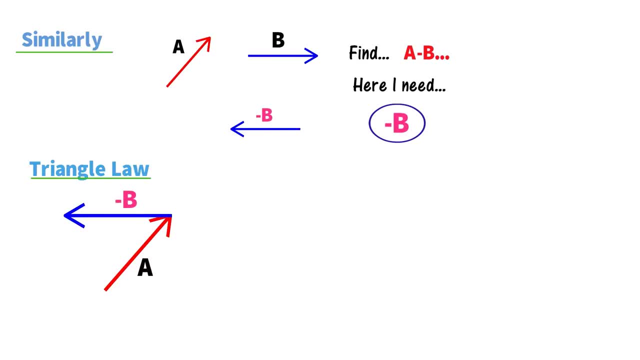 the negative of minus b, the negative vector of b, and that is, and this direction, and i will join the tail of the vector b with the head of the vector a. now, to get the result of these two vectors, or to get a minus b, i am joining the tail of the vector a with the head of the vector b. 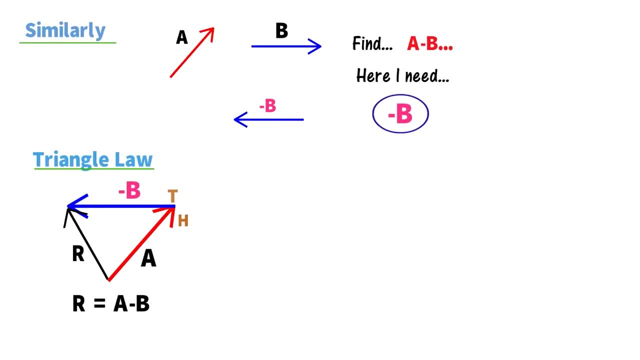 and i am getting r is: r is equal to a minus b. now this is the vector subtraction by triangle law. now i can also find out the vector subtraction by using parallelogram law. now, first of all, i will take the vector a and then i will take the negative of b, the negative vector of b. 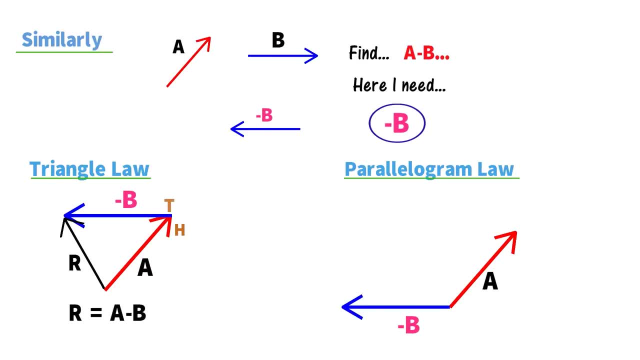 and I will join the tail of negative vector b with the tail of the vector a and I will get the resultant vector and the resultant vector. the tail of the resultant vector will be joined with the tail of vector a and with the tail of negative vector of b, and this is the negative. 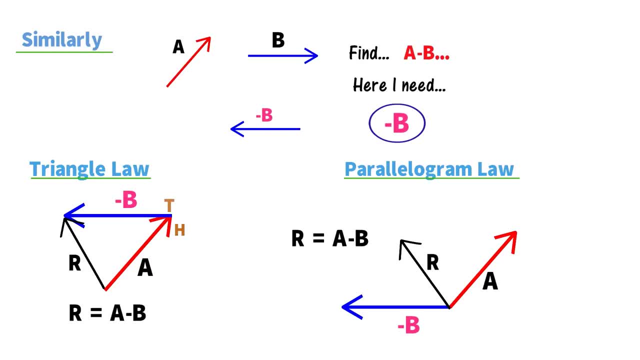 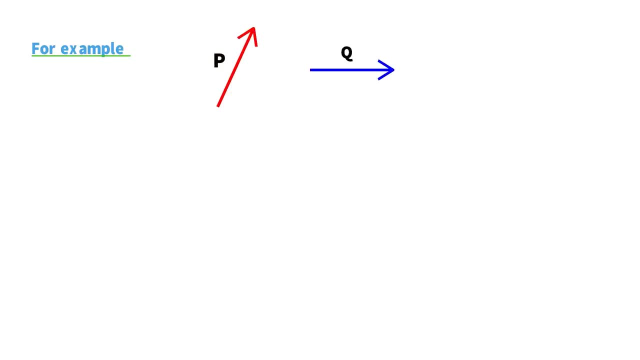 the subtraction of two vectors using the parallelogram law. now, for example, if I have another two vectors, p and q, and if someone is asking me to find out q minus p, now here I need the negative vector of p, and the negative vector of p is like this: now I can find out the. 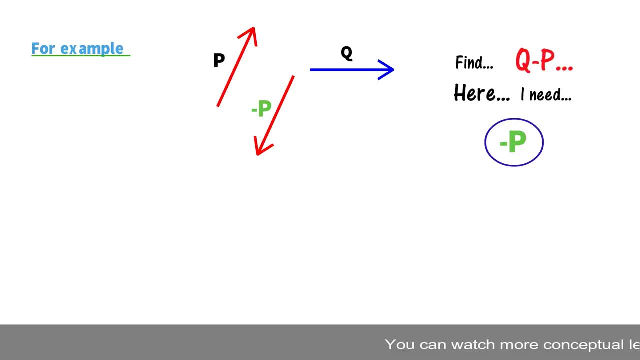 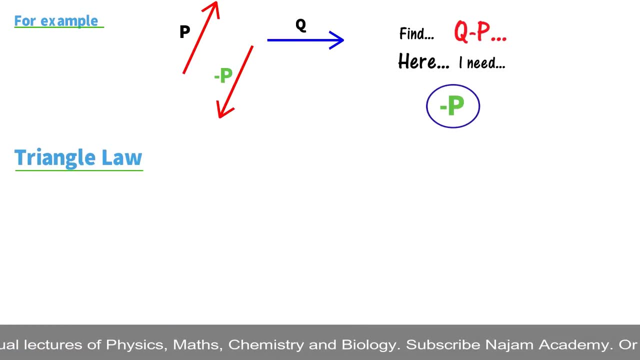 subtraction of q minus p by using two laws, by triangle law and by parallelogram law. so first of all I will use the triangle law, now I am taking vector q, and I will use the triangle law, Q, and, and then I am taking the negative vector of P and the tell of negative. 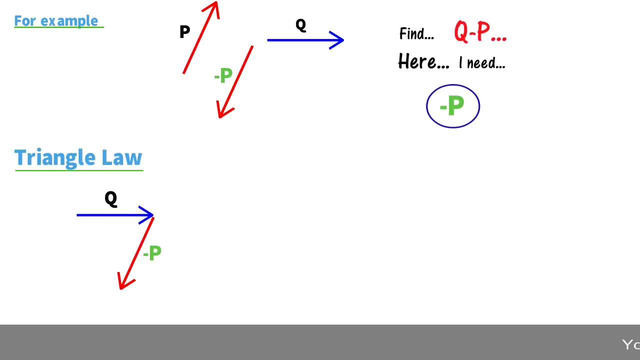 vector of P will be joined with the head of the vector Q. and now to get the resultant vector, I am joining the tell of vector Q with the head of the vector P and this is the resultant vector, and this vector is giving me Q minus P. now to find out Q minus P using parallelogram law, now, first of all here: 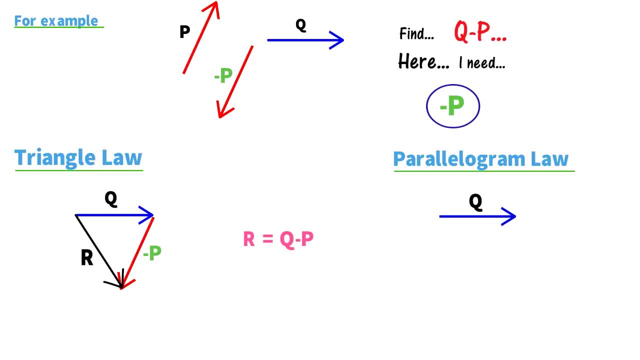 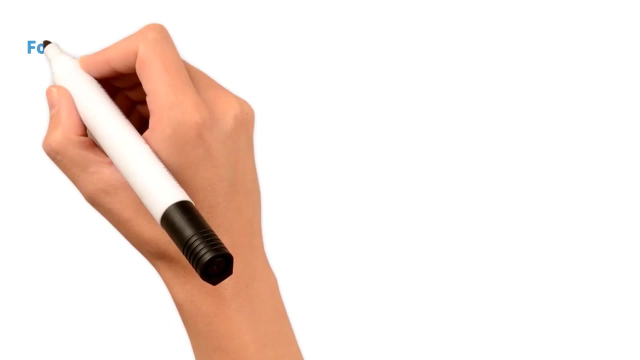 I will take the Q vector and then I will take the negative vector of P and the tell of negative vector of P will be joined with the tell of the negative vector of Q and I am getting resultant vector, and resultant vector is giving me Q minus P. let me tell you why vector subtraction is not commutative, for 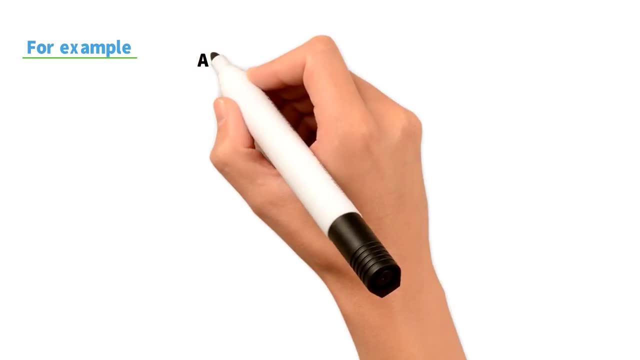 example, if I have a vector a is equal to 2i plus 3j, and if I have another vector b is equal to 5i minus 7j. now here, if someone is asking me find a minus b, remember here I need negative vector of b and the negative vector of b. 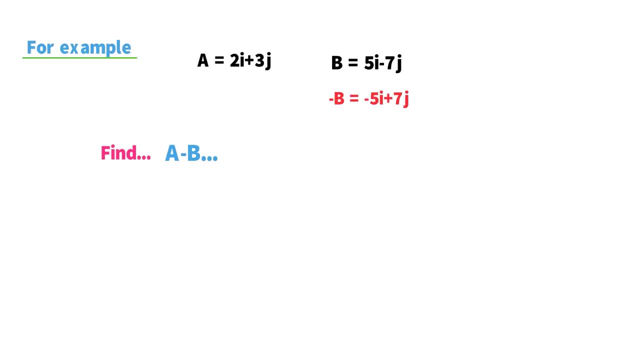 is minus 5 plus 7 j, and here I am finding out: a minus B is equal to 2i plus 3j minus 5i plus 7j, and I am getting: a minus b is equal to minus 3ラ. and I have another vector: b is equal to. 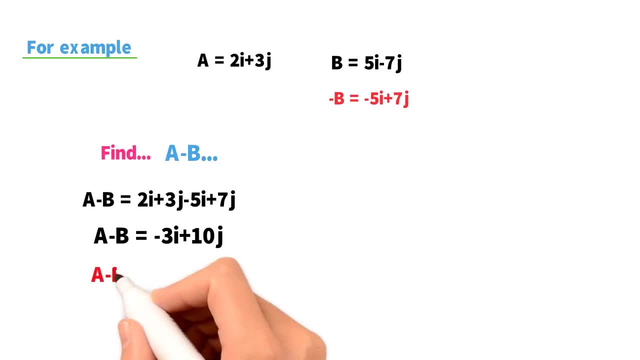 i plus 10 j and a minus b is equal to- and i'm taking minus as a, as a, as a common, and i'm getting 3 i minus 10 j. now, if someone is asking me to find b minus a, remember here i need the negative. 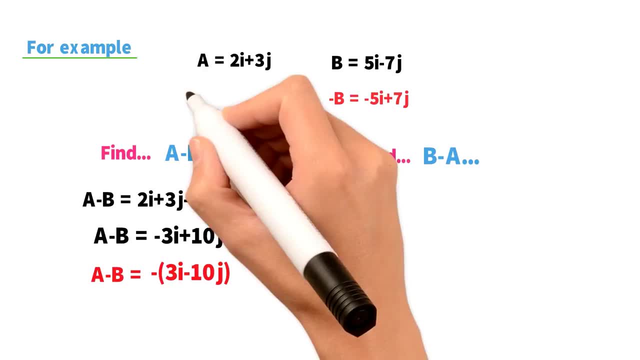 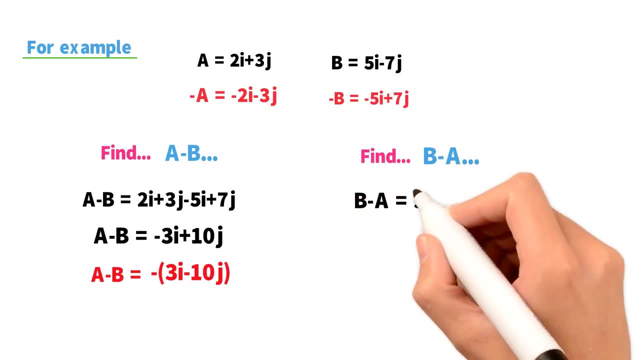 vector of a and i'm and i'm getting: minus a is equal to 2, i minus 2, i minus 3 j and b minus a is equal to 5. i minus 7, j minus 2, i minus 3 j and b minus a is equal to 3 i minus 10 j.